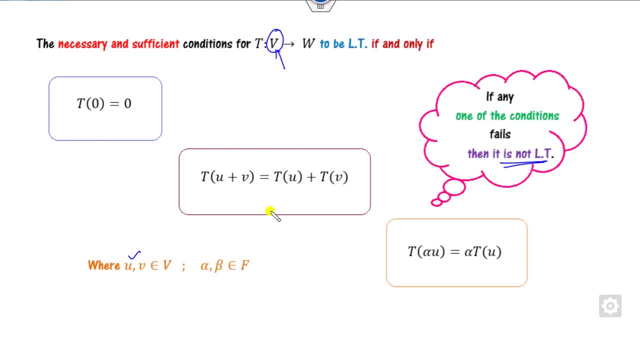 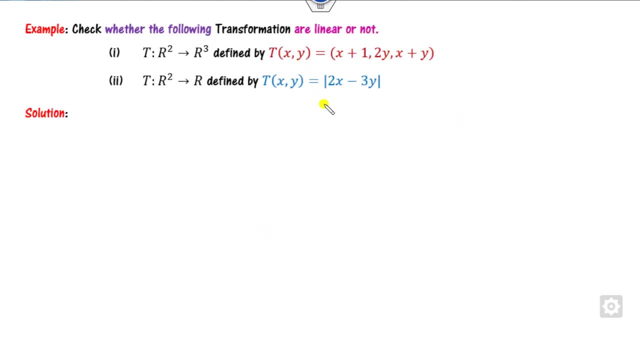 are from your vector space v, alpha and beta. that is, if there is only one alpha, then this alpha belongs to the field f, For example, if you look about there. so if you have to check whether it is a linear transformation or so here this is a r cube. 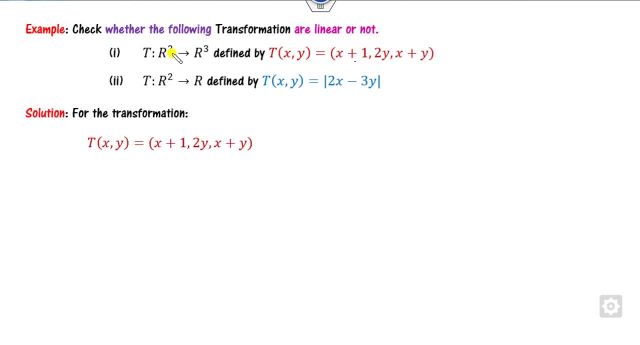 r scale. sorry, So you have to take the two elements for this first transformation from the domain So I can consider the two transformation as x1, y1. and second vector is my x2, y2, b2, both belongs to the my vector space r2.. Then you can clearly see that the first property of the 0,. 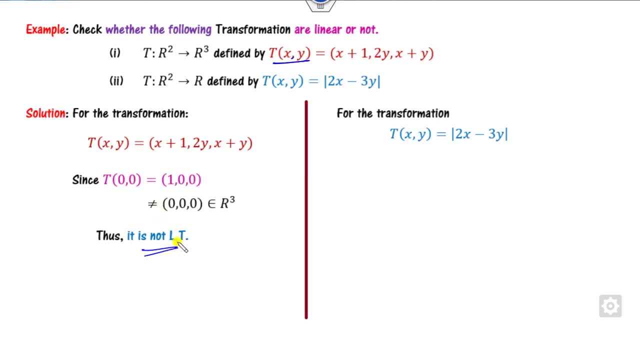 0, it is not be a 0,. it means this is not a linear transformation. So you have to just simply provide the one counter example if it is not a linear transformation. Second example is here. all of you know that whatever the mod of x is, this mod x is a linear or non-linear. So it is. 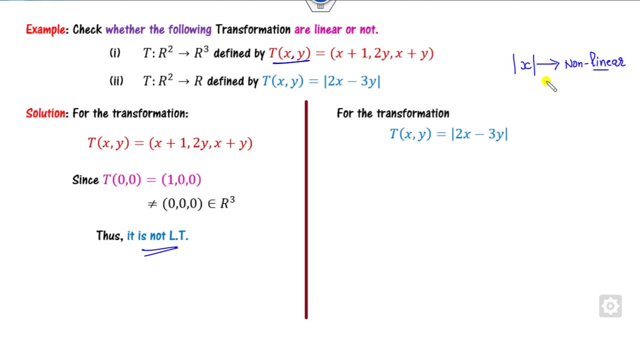 non-linear. Now, since it is a non-linear, it means it is not a linear transformation. It means we have to provide the one counter example. You can clearly see that t of 0, 0 is my 0. So that first. 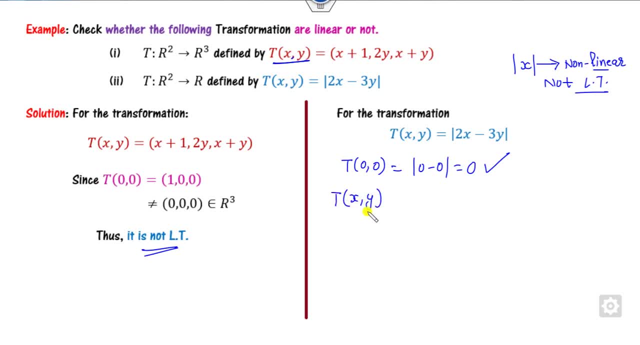 property is satisfied. So let us start with the x- y. So that is, you have to take the two elements- one is the u, second the v- from the domain r. Then you can start the t of u plus v. You can. 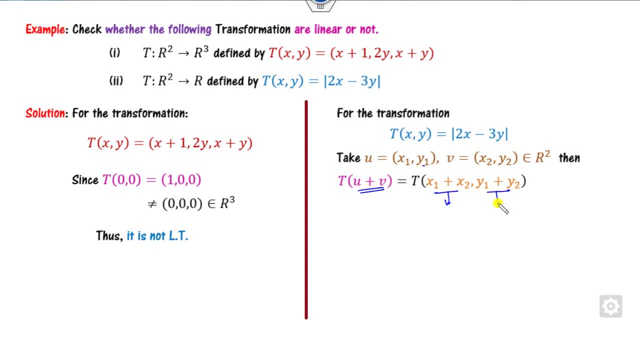 add them. you have to here. Now, this is my x, this is my y. you can substitute here. So it is 2x minus 3y. I can write this element as of 2x minus 3y. So this is my x, this is my y, you can. 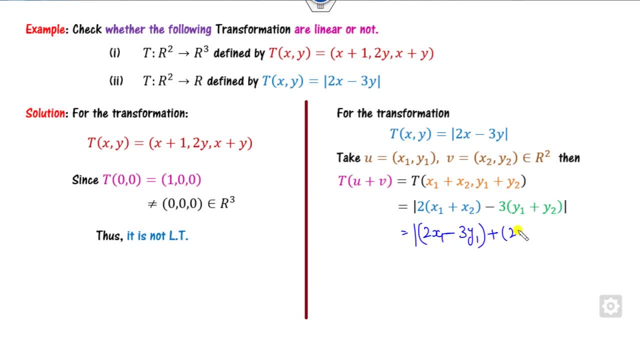 minus 3y1. I can take the first pair plus 2x2, minus of 3y2.. Now can you say this: what is the value of the mod x plus y? It is always be less than equal to mod x plus mod y. It can never be. 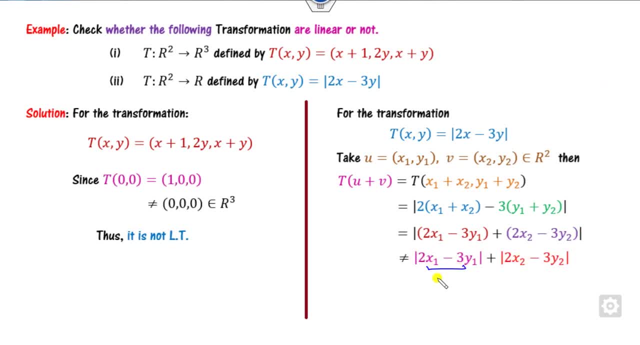 equality. It means it is not equal to this. because what is the meaning of that? This is nothing but x1, y1.. What is that? This is nothing but x2, y2.. What is that? x1, y1 is a u, That is. it is not. 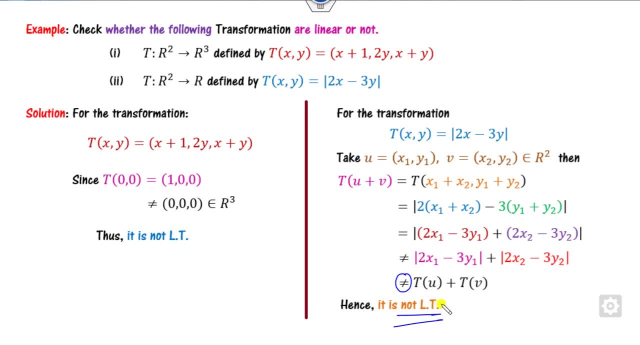 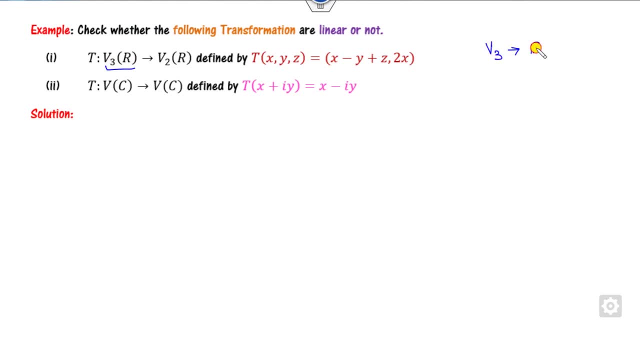 equal to So once it is a not equal to it means it is not equal to, So once it is not equal to it is not a linear transformation. Look what another one is there. Again, this is the v3.. What is the meaning of the v3?? This is nothing but my r3.. So again, first part is that you can easily. 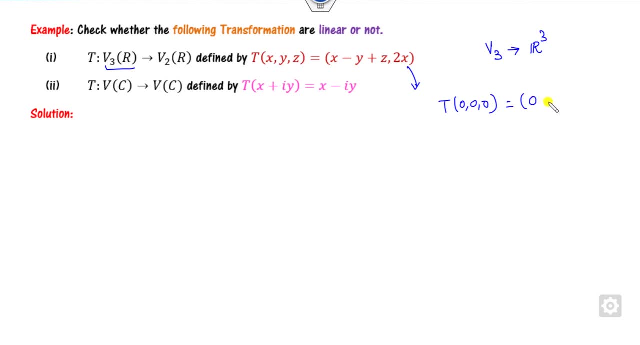 verify that whether the 0,0 is satisfied. So you can see 0,0.. So it is a 0, that is the first property satisfied. So we can also see that this value and this value all are the linear. So it. 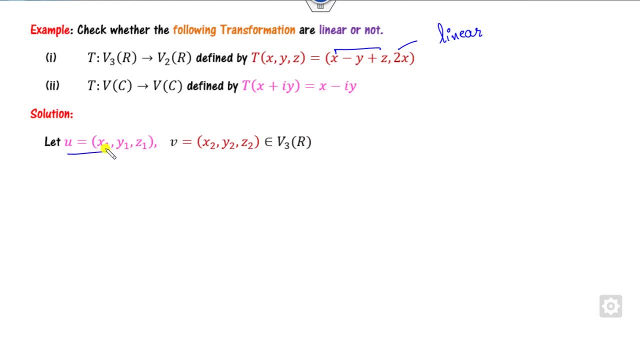 may or may not be the linear transformation, So I can consider the two elements from this v3.. That is, x1, y1, z1 and x2 are here. We can start with the u plus v and alpha u, If either. 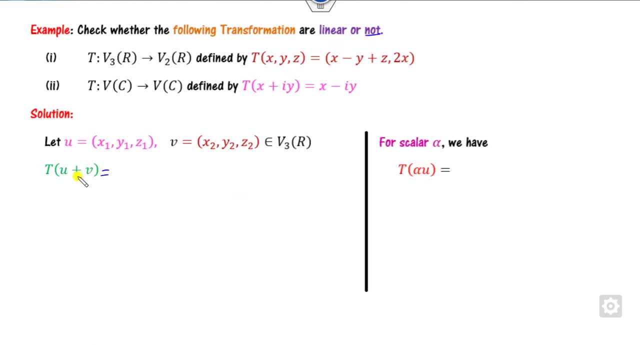 of the properties satisfy, then it is a, not otherwise. here, What is the value of the u plus v? And all of you know that whatever the u plus v, it is, also belongs to the v3 of r. Now you can start from here. Now, this is my x, this is my y, this is my z. I can substitute here x minus y. 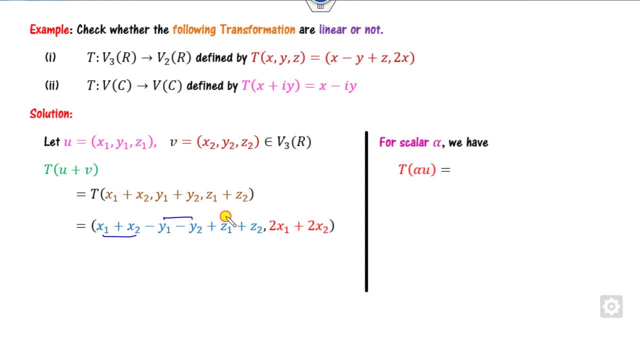 plus z. This is my x, this is my y, this is my z, and 2 of x. this is my z. Now can I write this, as I can combine them for the first pair, Like of here. So we can write: like here: This is the first pair and comma of the first pair are here. So what is? 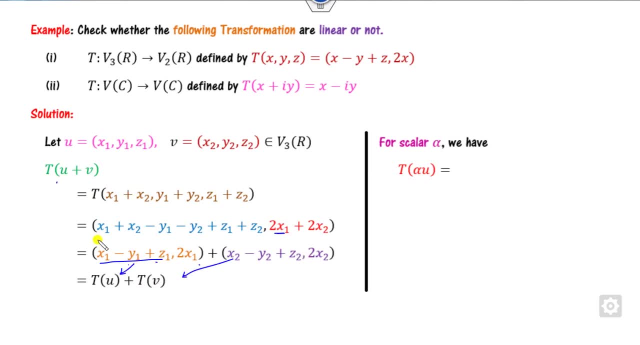 that This is nothing but the t of u. This is nothing but t of u. It means the first property satisfied. Similarly, what is the alpha of u, Alpha of u? nothing but the alpha x1,, alpha y1, alpha z1.. I can substitute this value again here. I can again take them. I can take this value as: 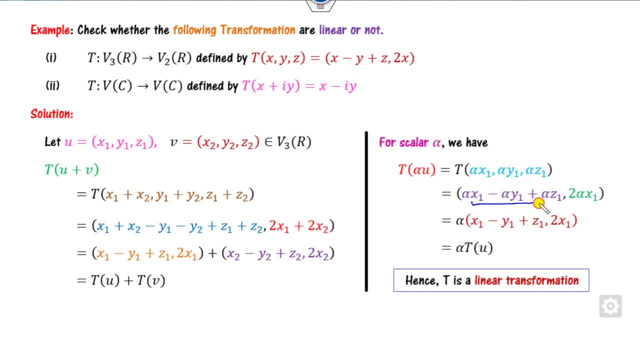 alpha common. So what will happen? I can substitute this value again here. I can again take them. I can, if you take as alpha common from here, alpha common from here. What is that? This is nothing but the? u, Since both the properties are satisfied. so it is a linear transformation. Or instead of 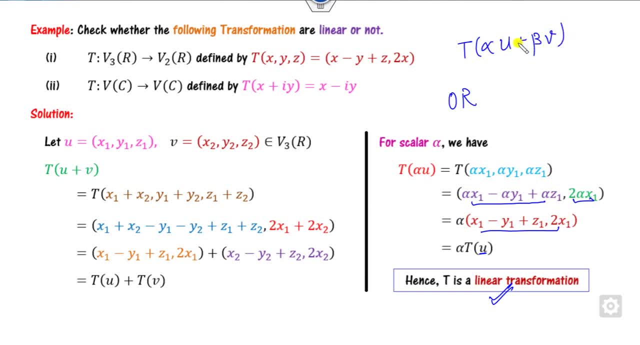 two properties. you can start from here directly, So like here, if you look for the second example. so our target is to show this one. Either you can show this property or you can show by two properties separately. I can take the elements from the v of c. That is a complex. 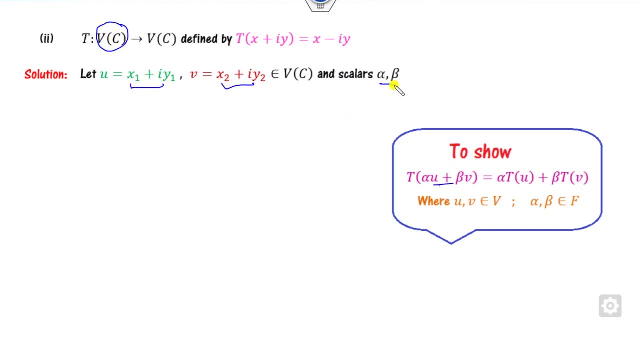 domain. So I can take an s here. Then, for any of the scalars are there. we can start from here. This is my x, This is my y. So what is the function? It is x minus iota y. I can write here. I can take the pair of the x1 and the. 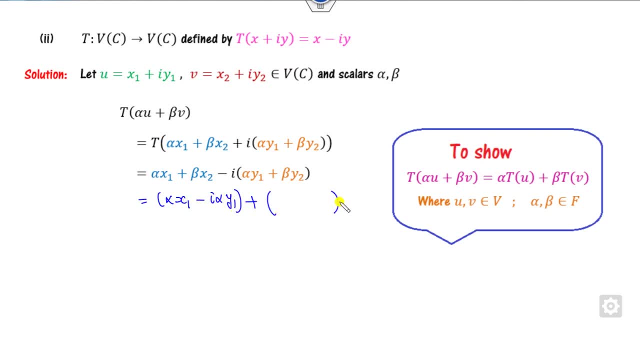 iota y of this plus of the second component. Now what is that? This is nothing but my here. This is x1 plus iota y1. That is t of u. So since this property is satisfied, it means it is a linear transformation. 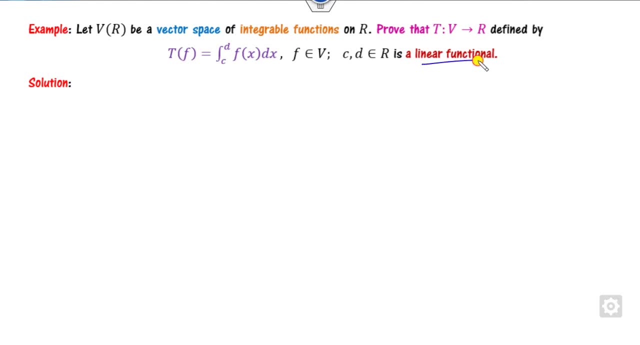 Look at the next example: are there? Can you say this is a linear functional. So again, you have to take the vector space from the v. So there is a function. are there? So I can take the two function, f and g. Alpha and beta are the scalar. Then you have to start from the here. 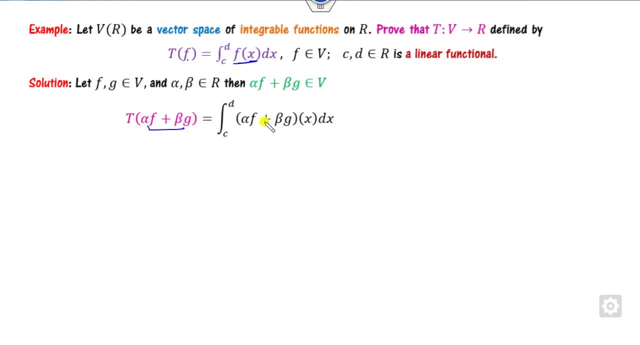 Now I can substitute the value of the f instead of here. I can open this bracket. I can write: here. I can integrate this by parts. Now I can take alpha as a common. Beta is outside. So what will this be? So this is so of alpha. this is g, which is my linear function In this. it means, since this is: 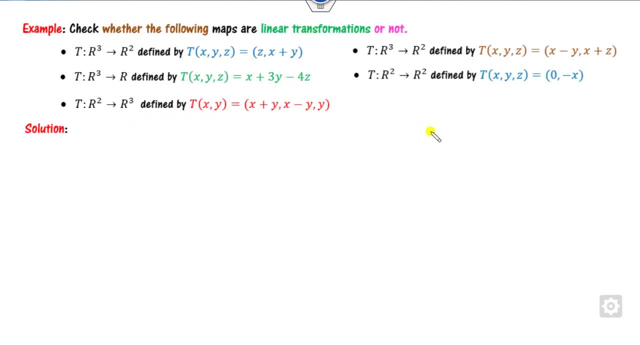 a zero and this is a zero. you can write it as aaterial function. Then from there the t of alpha. this is a Ç, So it is G, This is the t of alpha, t of G. It means this is nothing but my linear function. 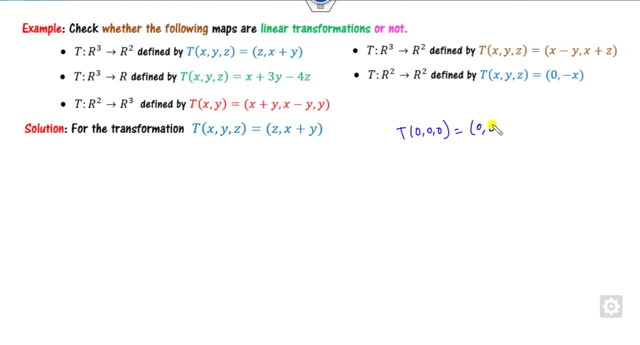 Look where these 5 examples are here. Firstly, you have to check whether any of them is non linear. Say, for example, the first part can be 0,0. satisfied, You can see it is a 0,0.. It means this is: 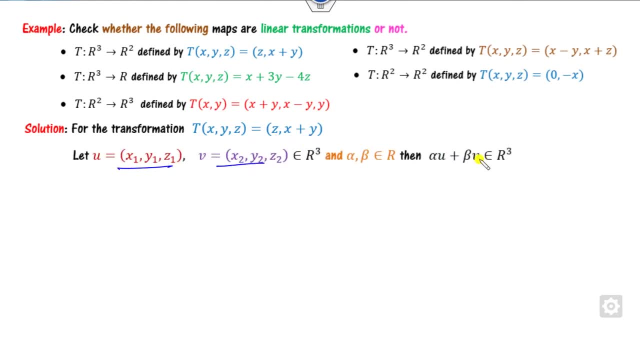 a satisfied And also this: a linear function, x plus y is also with the linear, So it means we have to check these properties. Do you remember solved? Subscribe Now. we anecdotes like this and you are not sure whether to learn. Please follow me on Twitter, Facebook and Twitter. Leave a Incom alkikv. 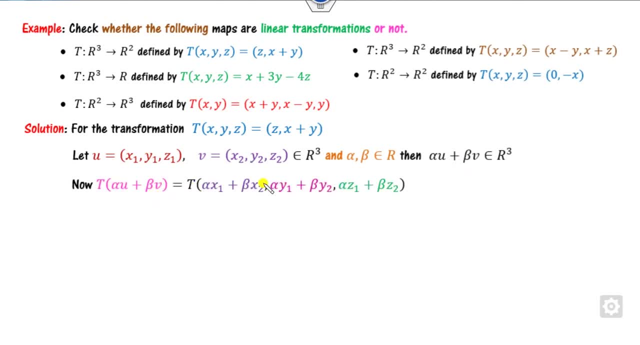 can start with the alpha u plus beta v. so once you will start from the alpha, this is the x, this is the y, this is the z. so this is z, this is y and x. i can substitute here z, x plus y. now i can take the pair of the z one. this is x one and this is the y one. i can write this one: this is the pair. 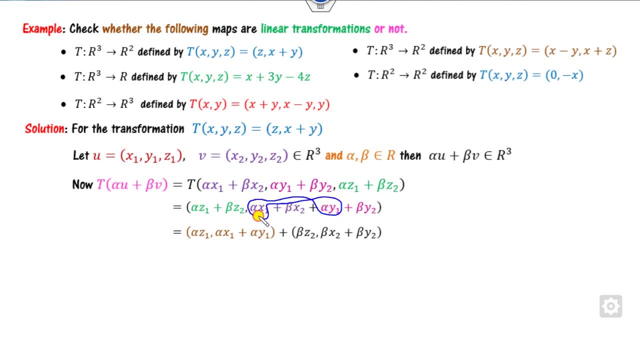 of. i can take the pair of this and rest r. what is that? i can take alpha as a common. what is that? this is nothing but my. this one, that is x one, y one, z one. this is my, nothing but u. so this means this is a linear transformation. look at the second one out there. so if you start from here again, you. 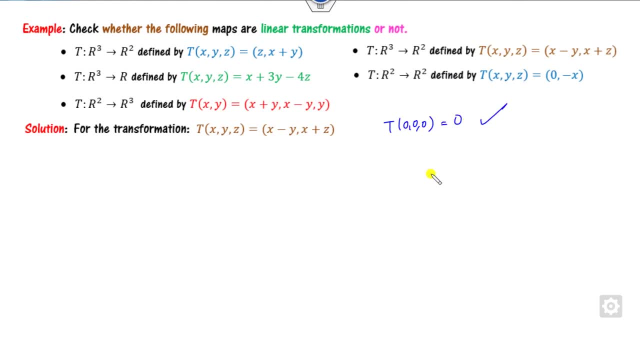 can see the zero comma zero. comma zero is zero, that's a satisfied. so we can start from the here again. so we can take alpha u plus beta v, which is nothing but here. in this case, this is my x, this is my y, this is my z, so i can substitute here x minus y and x plus z. 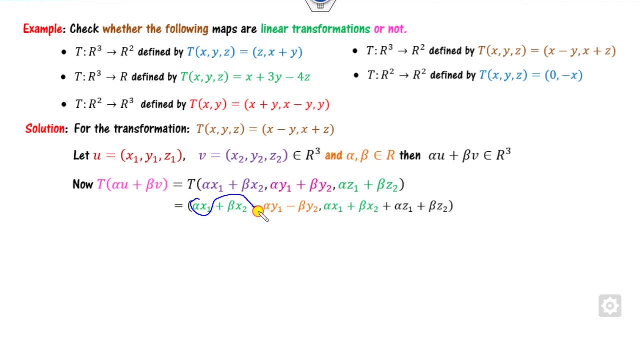 now again, i can take the pair of the one that is a. this is the first pair and from here, this is my first. i can write these elements as of here. so this is this pair and this pair. i can write, like i can take alpha common from the first part, beta common from the second part. 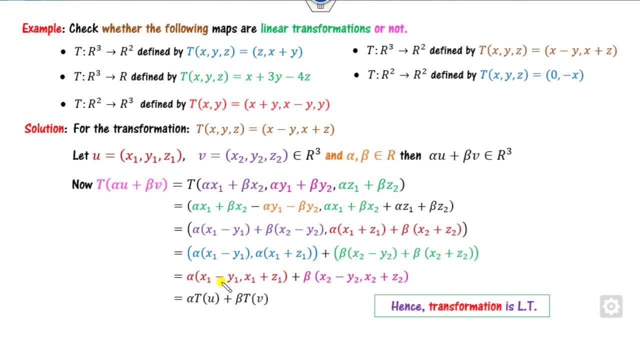 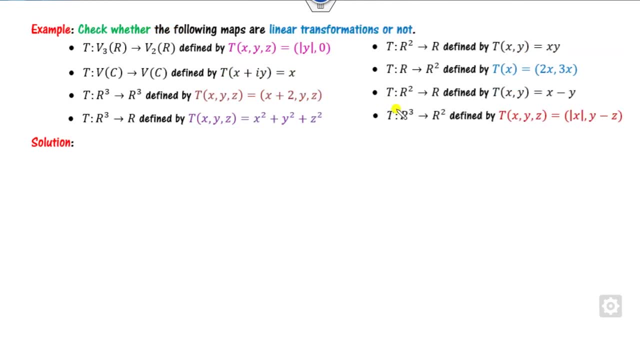 and this is nothing but my t of u. second is t of v, rest part. you can easily verify by yourself- now look about that- whether it's a linear or non. look at that. if you consider this function, clearly see that it's a non-linear. so it means this is not a linear transformation. 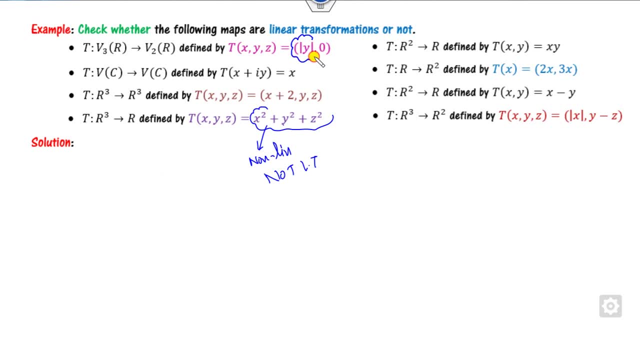 so you have to provide one counter example again. you can see: this is a mod x, this is a non-linear, it's not a lean, it's not a linear transformation. x, y, what is the degree of this? the degree is my two. it means this is not a linear transformation. the here. the degree is one. it may or may not be. 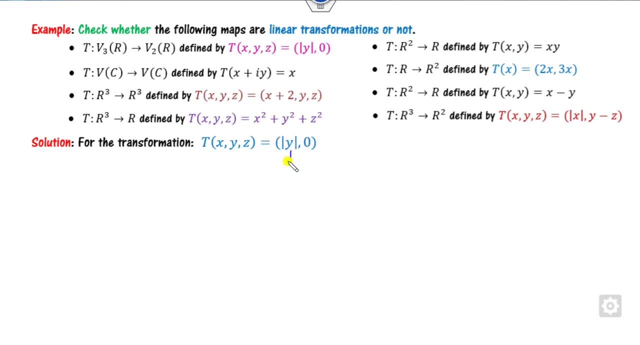 and so on. so let's start with the first part, since it is a non-linear, so it means this part is not a transformation, so it means you have to provide the one counter example enough. so let's start with the u and v, and we can start with the u plus v. this is my u plus v. what is that? this is the. 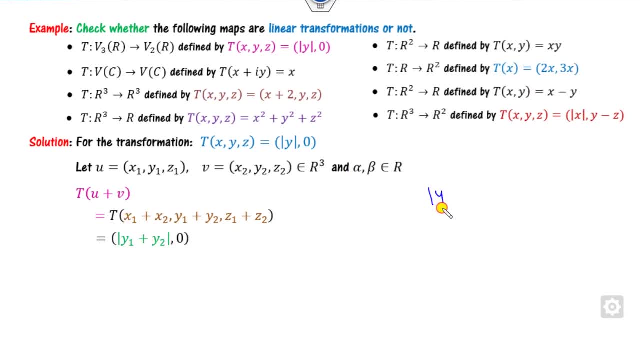 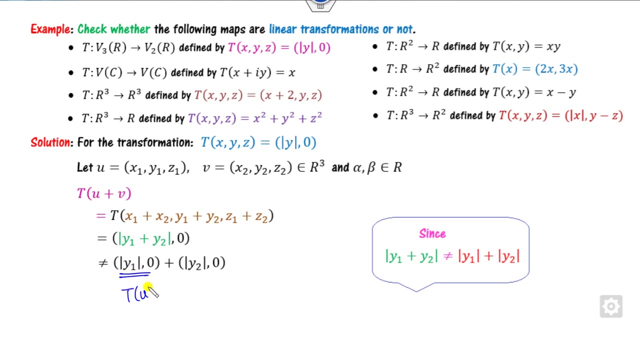 mod of y. so this is my y. now how you can expand the value of the mod x plus mod y. it is always be less than of mod here, but we need always an equality. so it means it can never be here because of this, so it can never be equality. so what is that? this is nothing but my t of u. this is nothing. 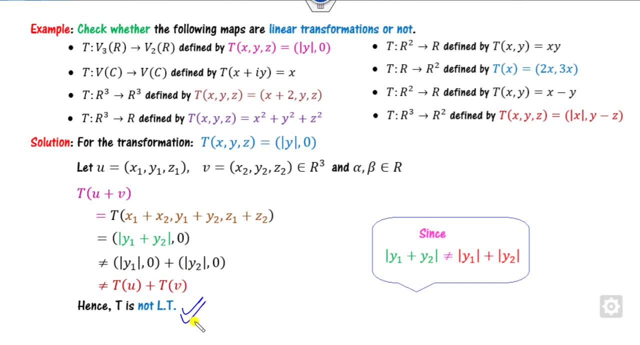 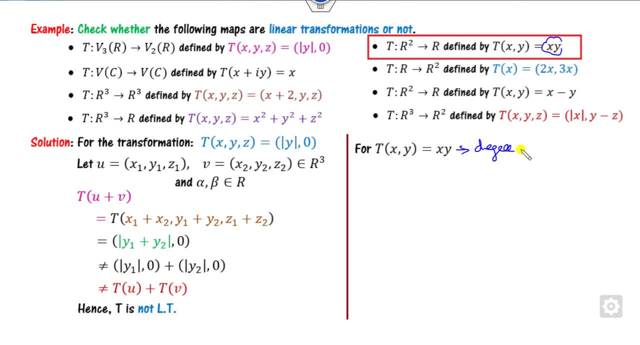 but my t of v. so since it is not a linear transformation, look about second one again. you can see what is the degree of this. you can see the degree is my two. it means it is not a linear transform. clearly see that if you start from the alpha of u and if you substitute the value of here, this is my x, this is. 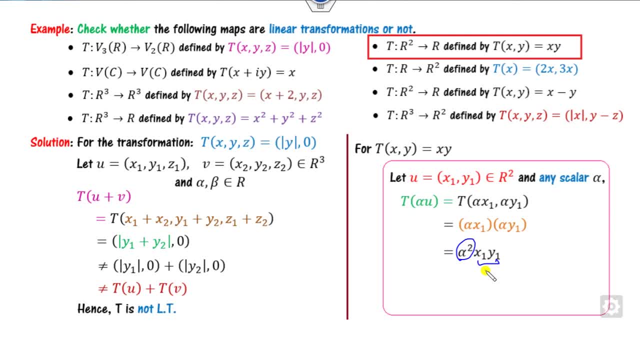 my y. it is nothing but my alpha square. what is that? this is nothing but my t of u, but we need is not equal to alpha. it means this is not a linear transform. or you can also start with u plus v. you can easily verify: these are not equal to t of u and t of v. look about these two. 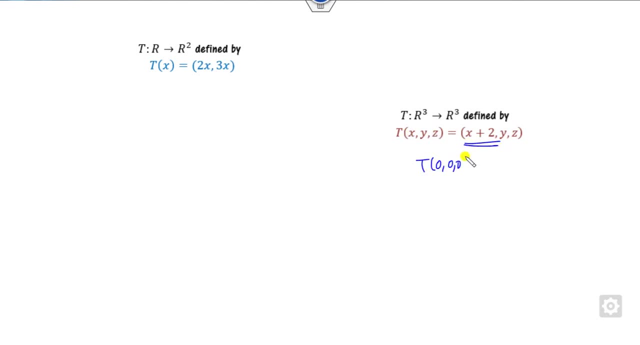 examples are there. clearly see that in this case it is a 0 comma 0 is not satisfied. it means this is not a linear transform. you can see: here is that 0 comma 0 satisfied. here is the element 1, so it is a 0 comma 0 which is satisfied. so it means we have to satisfy these two properties now here. 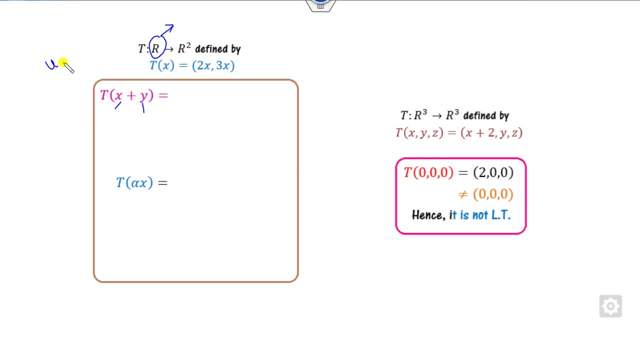 there is a r, so it means i have to consider x and y, or you can say u and v. so what is the value of this is? it is nothing but my 2x here. now i can take the pair of the x and x, y and y. 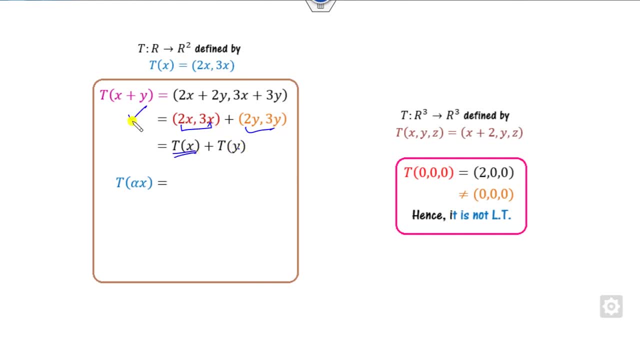 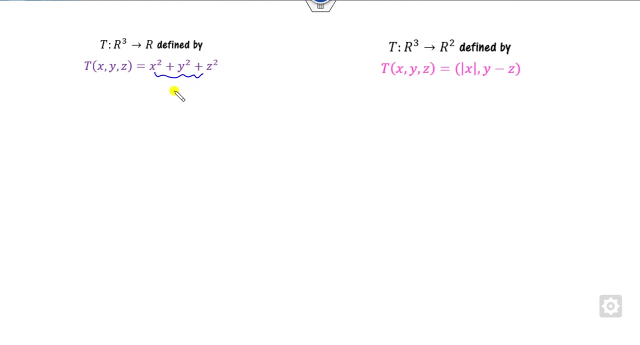 what is that? this is t of x. this is t of y, so it means this set is 5. look at the alpha of x. here i can take alpha common. what is that? this is nothing but my t of x. it means this is a linear transform. look for these two properties again. you can see. this is a non-linear. it means this. 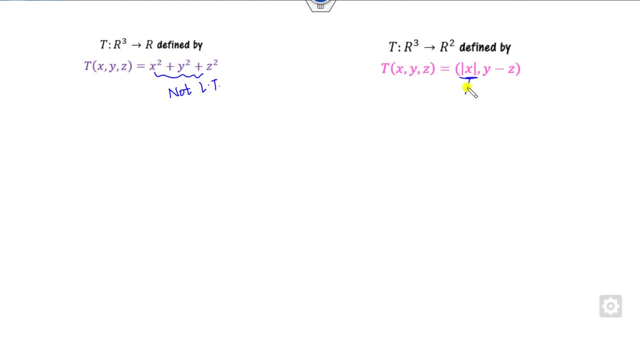 is not a linear transform. again, mod x is my non-linear function, so it means it is not a linear transform. so how you can prove that? you have to provide some one counter example. so say alpha of u: i can take this value into here. x, here i can take alpha. 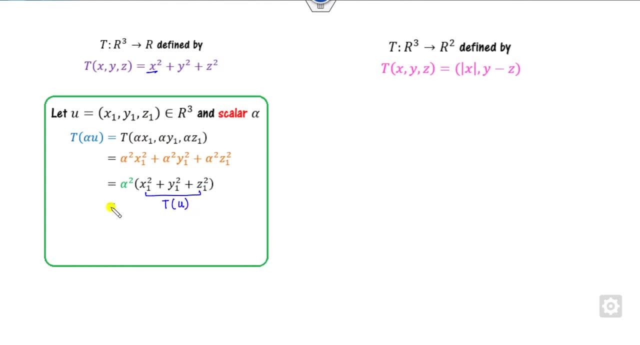 common. what is that? this is nothing but my t of u, but this is alpha, square time t of u. but we need always as alpha, which is not equal. it means this is not a linear transform. this is the mod of x. again, it is not a linear transform. you can start the u plus v. 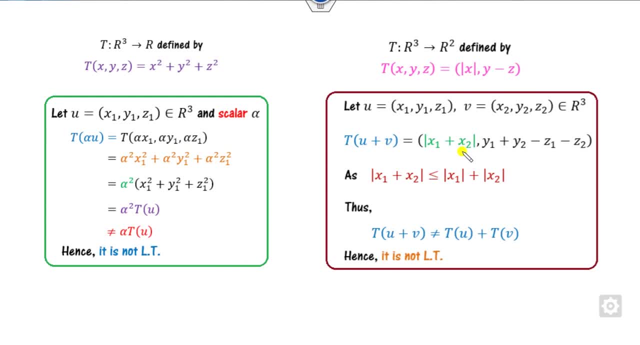 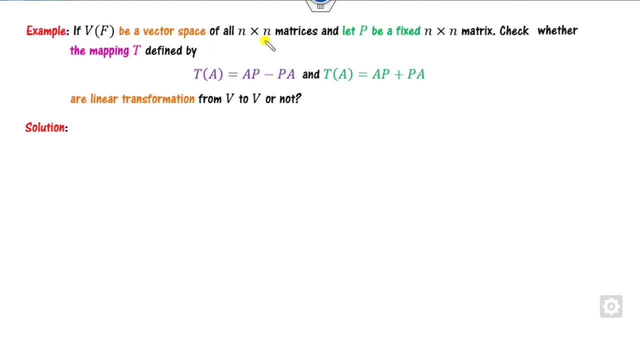 what is the mod of x plus y? it is always be less than of this, so it means this can never be the equality. hence it is not a linear transform. look at the another case. are there? if you consider the vector, space consists of the matrix. then you have to prove whether these are the linear transform or 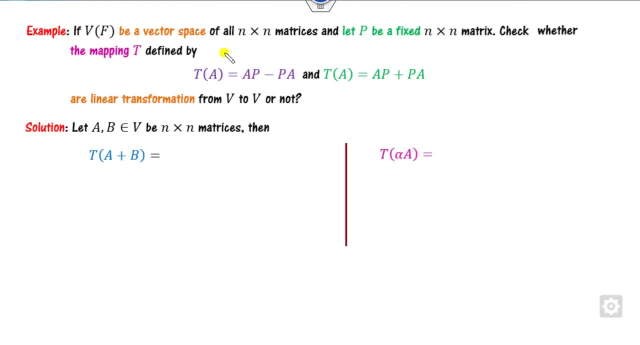 not now here. you have to provide the matrix, so i can consider the two matrix a and b of n cross n. we have to check whether these two properties are satisfied or not. let's start the first one. this is my a plus b. i can substitute here and remember. 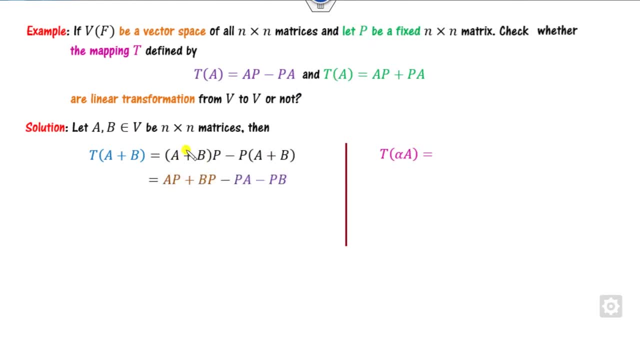 that p is my fixed. that's why it's a constant. now i can open this here. i can take the pair of this. what is that? this is a p minus p. this is nothing but the t of a. b. p minus is the t of a, so it means. 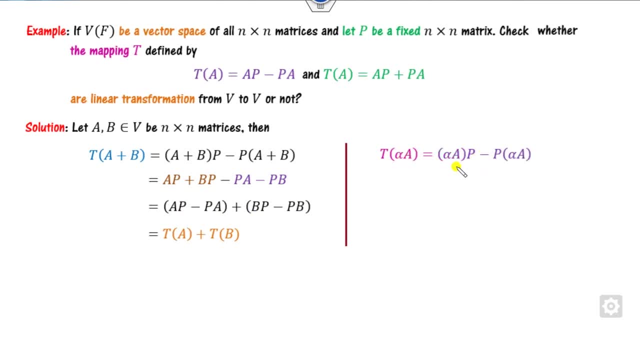 the first property is satisfied. similarly you can start with the alpha of a here. we all know that when you scalar multiply them it can be taken outside. so it's a, a of p, and here i can take alpha as a common. we will get here so clearly: see, is that both the properties satisfied? it means 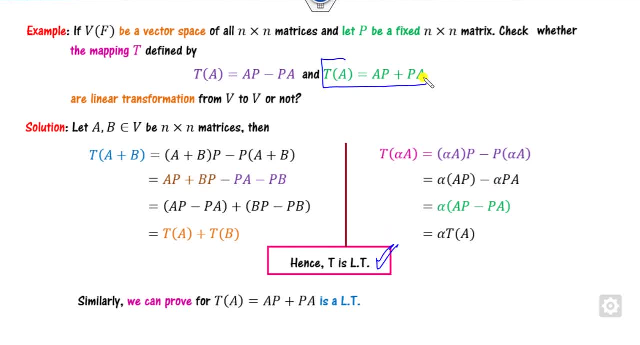 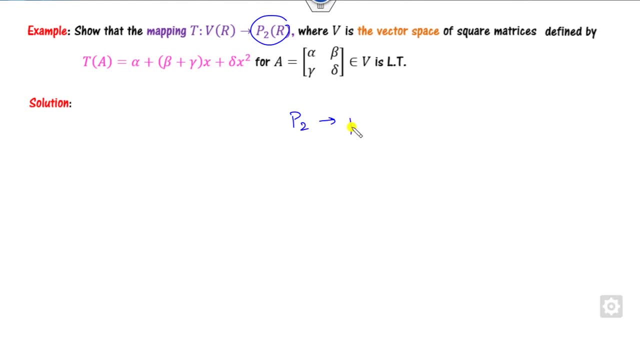 the linear transform- similarly- you can prove it by yourself- is here. look at the last example here. this is the polynomial. what is the p2? p2 is the polynomial of degree less than equal to 2, so it means you have to consider the a. what is the a is a matrix, so i can consider the two matrix. 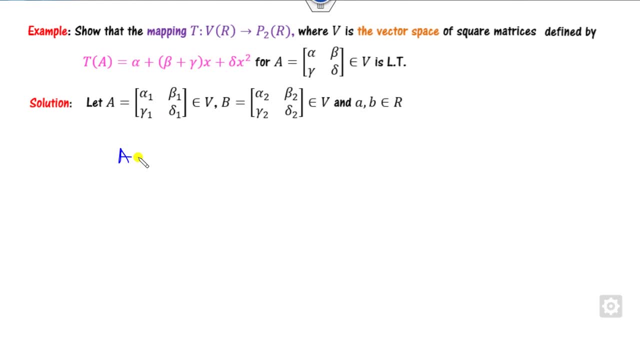 a and b of these elements, such that what is the value of the a plus b? or you can say alpha plus b already there. so i can consider here as a of a plus b of b. so if you take on them you can see again: this is a, 2 cross 2 matrix, so it means it belongs to the b. now i can start with the here. i 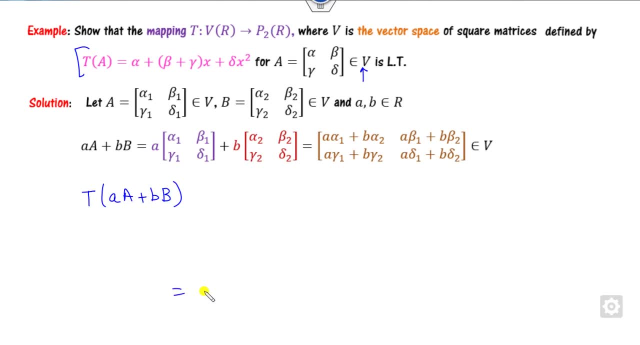 can start with this value, and my target is to prove whether this will hold or not. so what is that a of? so i can substitute this value. so this is the alpha you can see here. this value is my alpha according to this, so i can write the first pair. 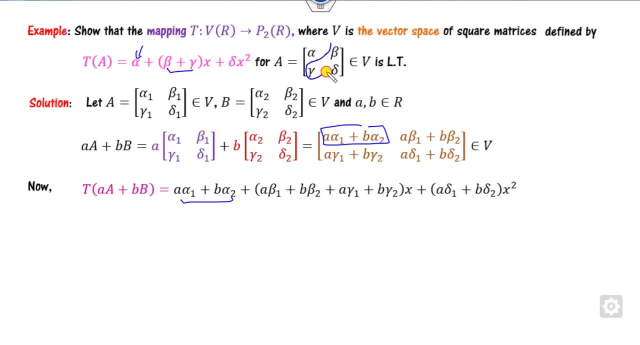 alpha. what is that? this is beta plus alpha. beta plus gamma, that is this value. so it means this, and here i can add these two values. and now, if you open this bracket, take the pair of the one, and so on, this is the pair of the x, and so on. so all these elements are with respect to the index. 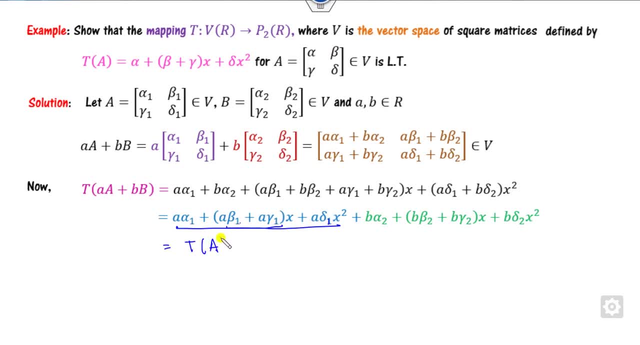 one. what is that? this is nothing but my t of a. sorry, i can take a as a common. firstly, what is that? if you compare this, this is the same thing. this is the index one, that is the index one and that is my here. it means this is a linear transformation, so this is the way you can.